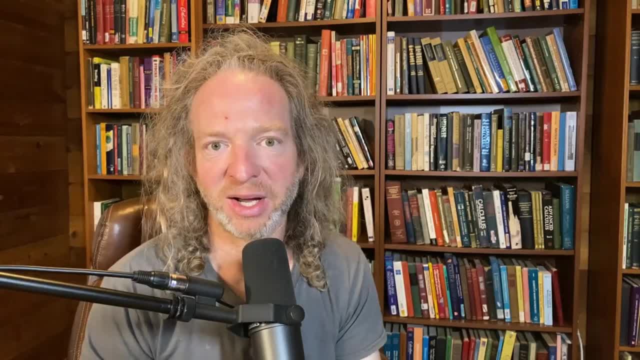 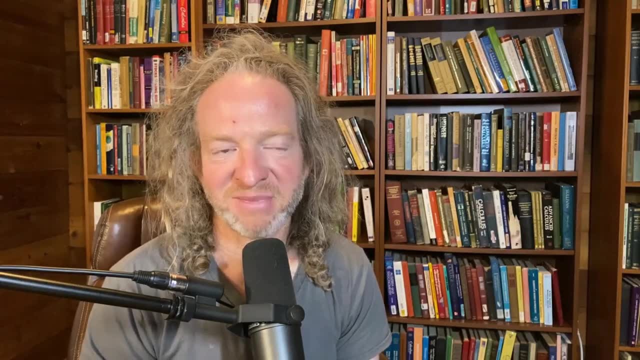 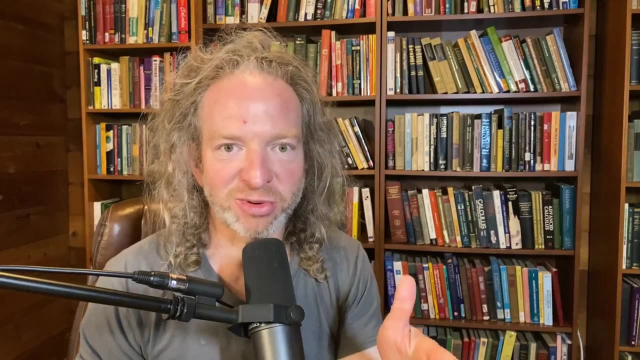 equivalence And I went in and I spoke to my college advisor. I told him that I wanted to get a PhD in computer science And he didn't laugh at me. He took me really seriously. He put me in this advanced class, which was basically pre-algebra and intermediate algebra combined. This person, Omar, 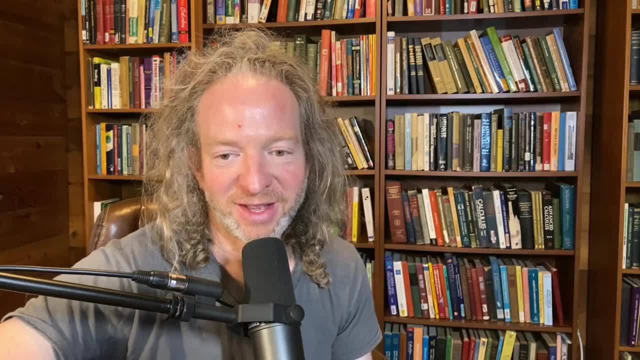 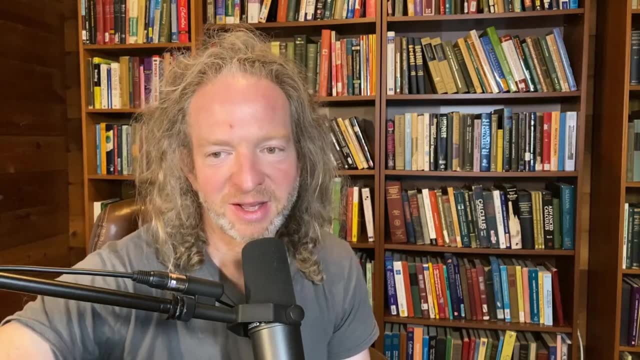 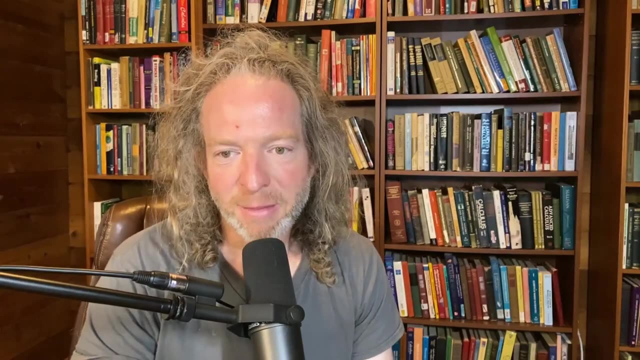 is taking intermediate algebra And they have a question that I think a lot of people would look at it and they would say, no, you're not ready. But I think Omar is ready. The subject is proofs writing. Hi math sourcer, I'm a big fan for you and for all maths and science. I am a very absolute. 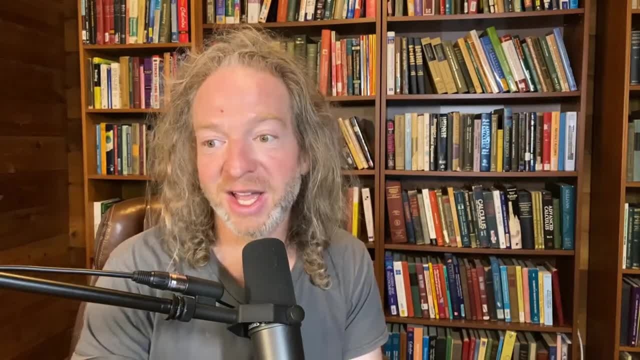 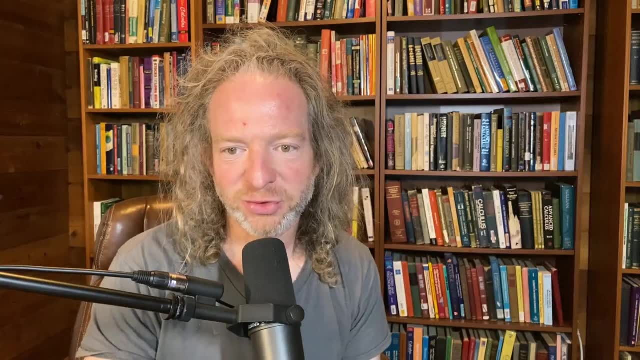 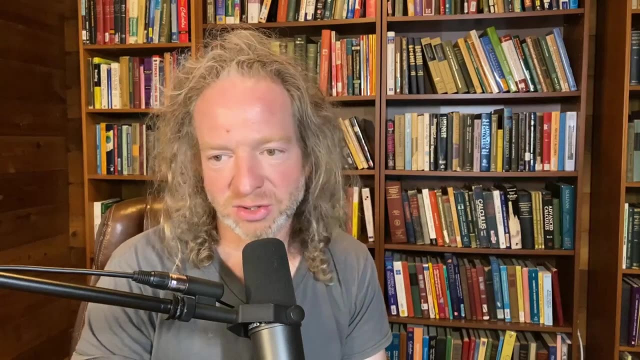 beginner and now I am studying intermediate algebra and I know about your roadmap and everything. So my question is: when should I start on proofs writing? Should I start right now, And do you think I should delay my decision? Should I wait until after calculus or something? Thank you, So here's. 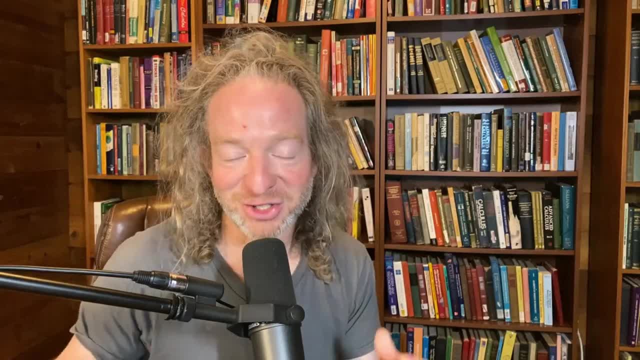 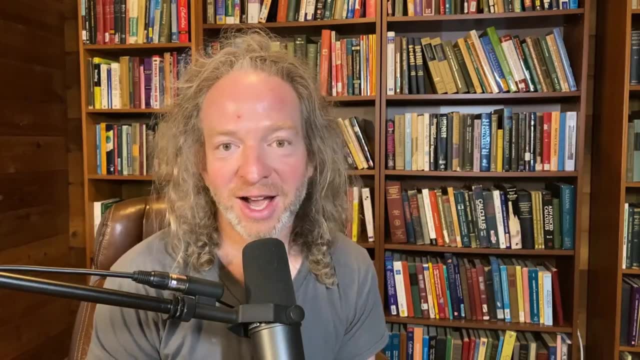 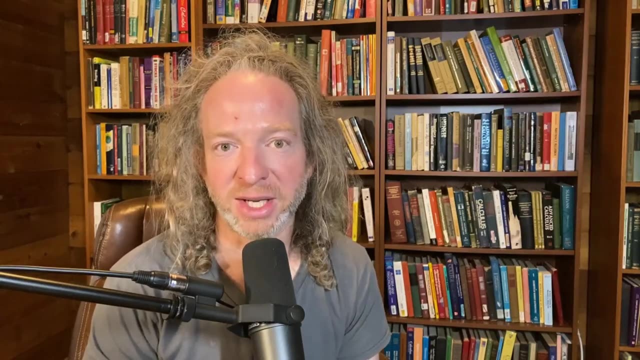 a person who is just getting started with mathematics- just like me, right? Just like me, just like I was Intermediate algebra- And they want to know if they can jump into proofs. I think the obvious answer is yes, Absolutely, Because the wonderful thing about proof writing is all you have to do is be able to. 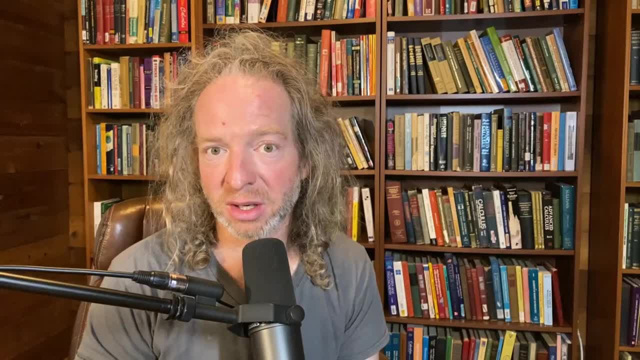 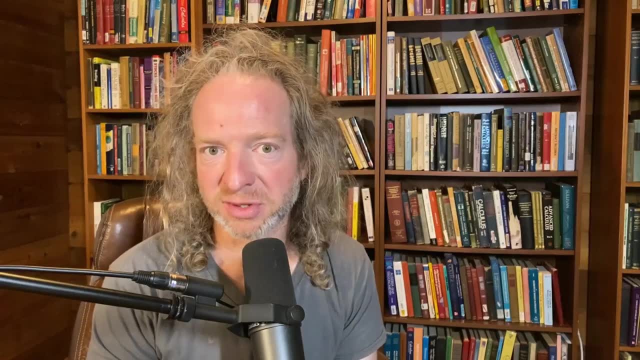 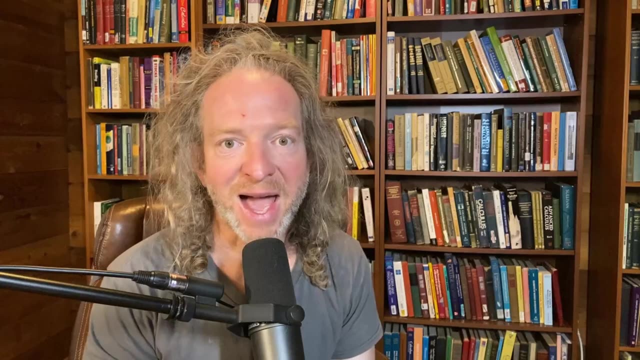 read And anything you can learn. anything you learn is better than nothing. I wish I would have started learning to write proofs much sooner than I did, Because once you learn to write proofs, you can get a math degree. That is what keeps people from finishing their math degrees. 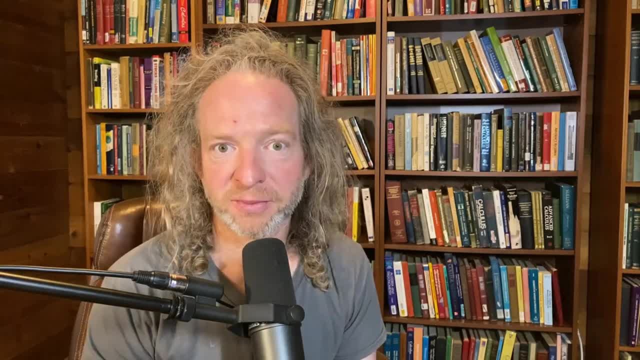 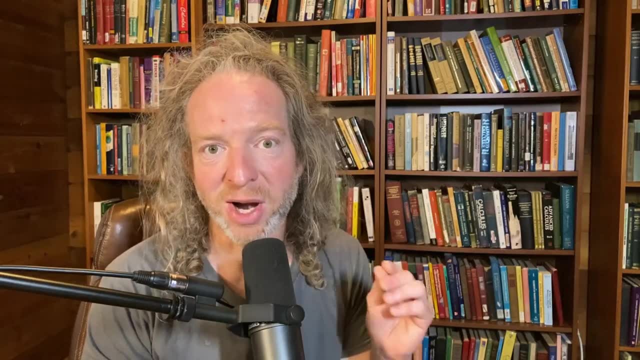 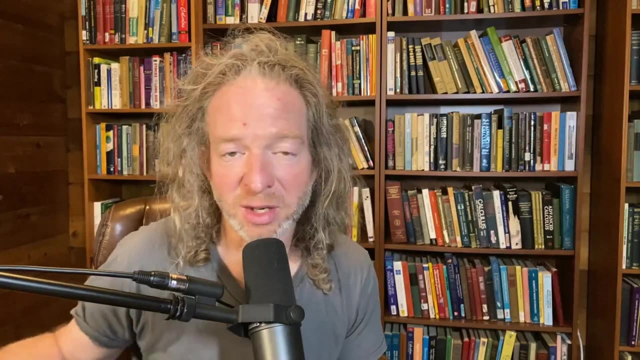 It's the ability to construct a proof. It is such a huge thing, It is such a huge hurdle. I was really lucky because I was able to take two proof writing classes at the same time, And I think that really helped me. So, Omar, I have a book here and I have a ton of books on proof writing and there's free ones on 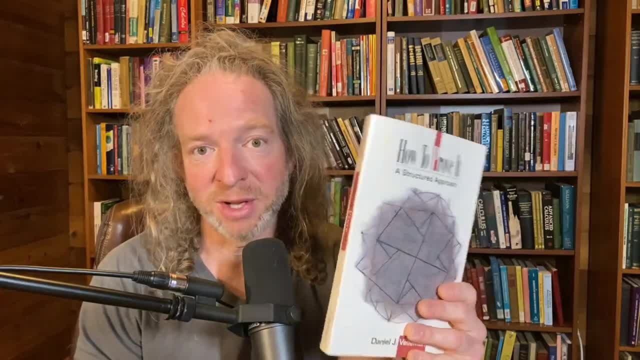 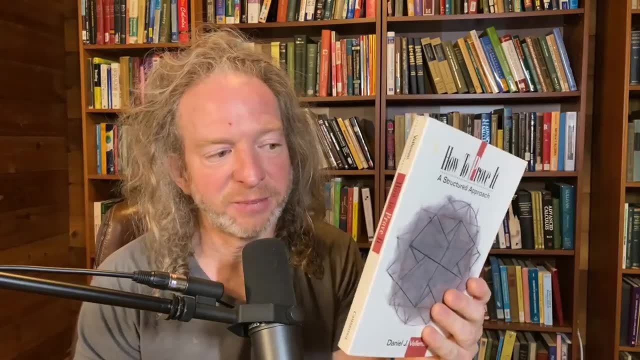 the internet, but I grabbed this one because it's one of the better ones in my opinion. It's also not super expensive. It's called How to Prove It- A Structured Approach by Daniel Velleman. This is a book that I did not want to buy. I did not want to buy it. I did not want to buy it. 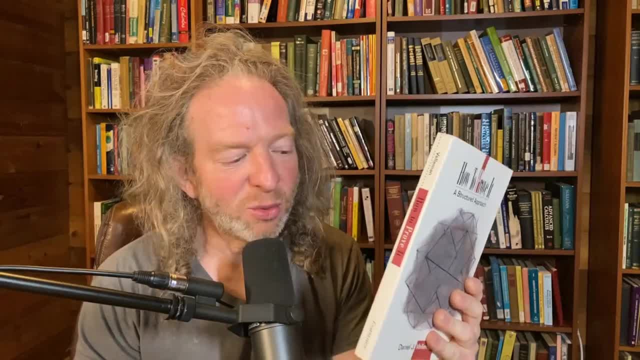 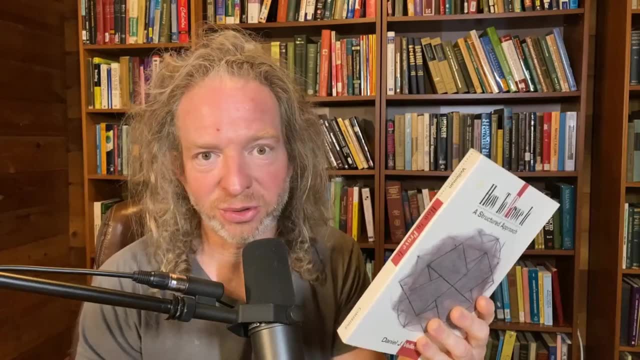 That's what makes this book even extra interesting. I didn't want to buy it for a few reasons. One, I felt like it was above my price range. I think I paid more than $20 for it. Two, I already had a bunch of proof writing books. Three, I didn't like that it was a soft cover. 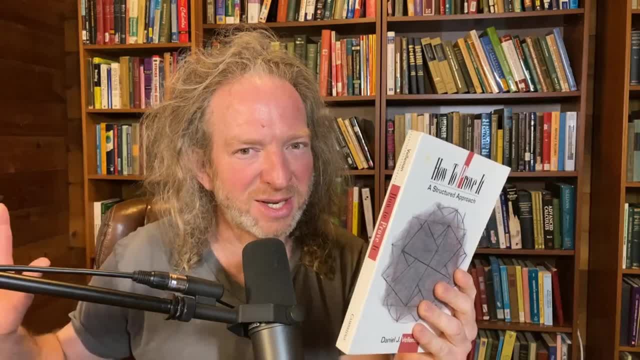 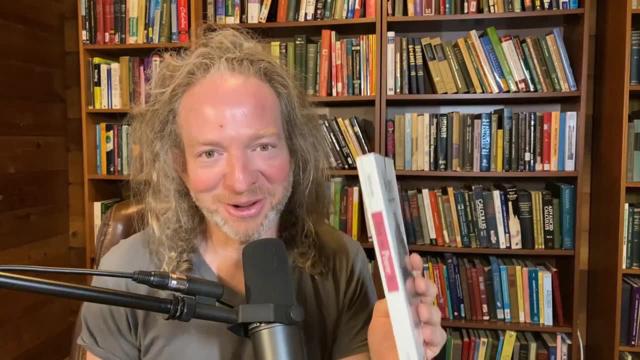 There might be a hard cover available, but that was, I think. if there is, it's a lot more, I think. But due to peer pressure from people here on the channel, I bought the book and I love it, I think. 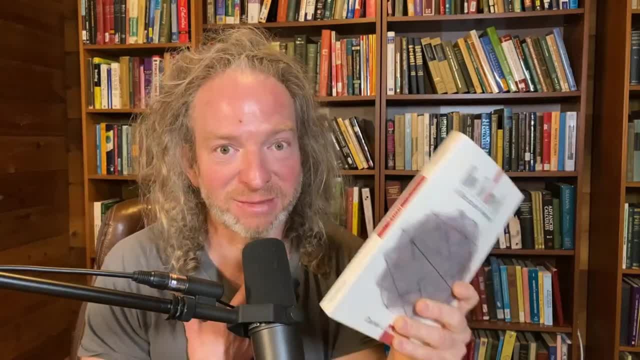 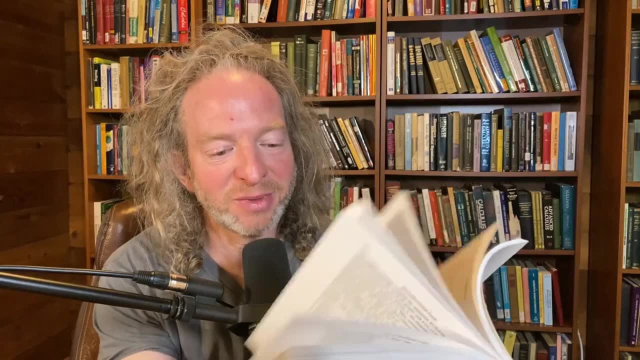 it's probably the best proof writing book, in my opinion currently. This is my favorite one currently, So that's why I'm recommending this one. I'll leave a link in the description, Omar, if you want to check it out. It does a great job explaining what a vacuous truth is. I've never 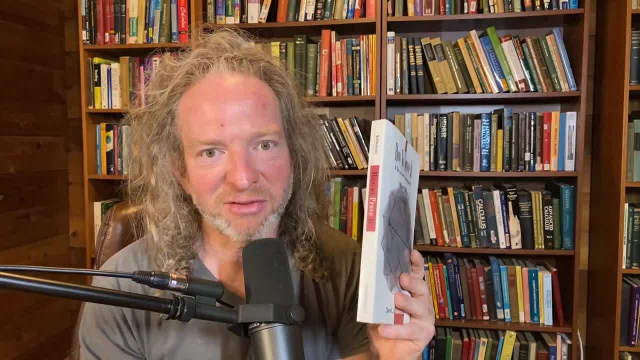 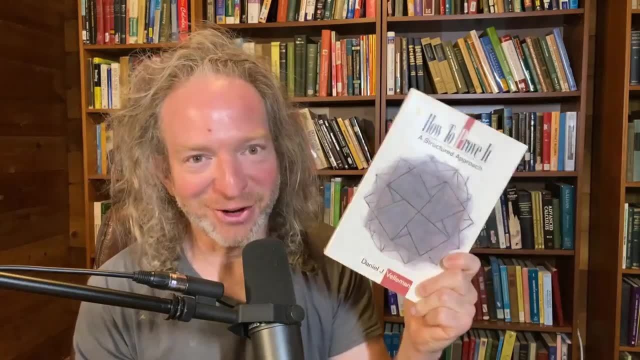 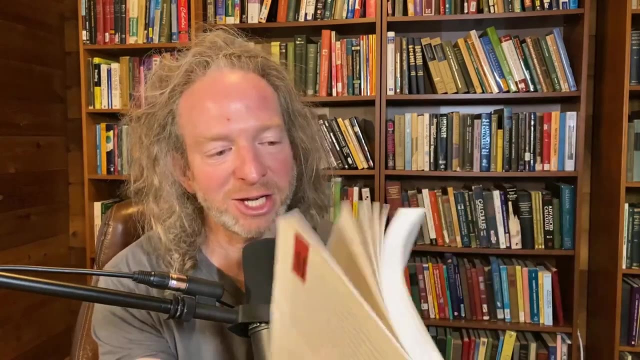 seen a better explanation of vacuous truths anywhere. I think Daniel Velleman does a superb job. I always wish I could get it autographed or something As a collector. you know it's a big deal. It's a big deal, But wonderful book. And just start reading. You know it starts from the 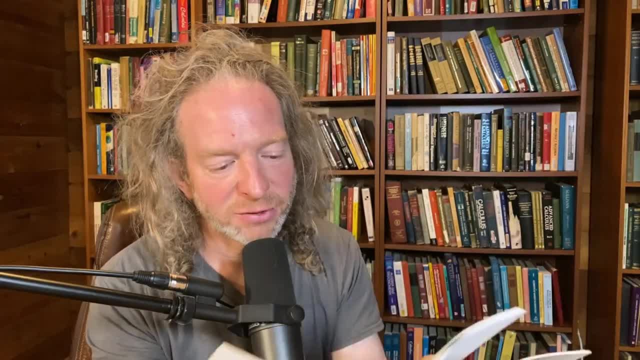 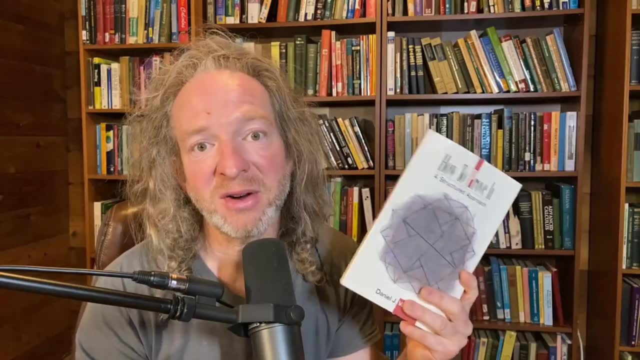 beginning. You can just get started with it. You might not understand stuff, It's okay, Just keep moving. It talks about, you know, statements and some of the logical symbols, And it's going to be very, very different from intermediate algebra. Now, many people are probably watching this and 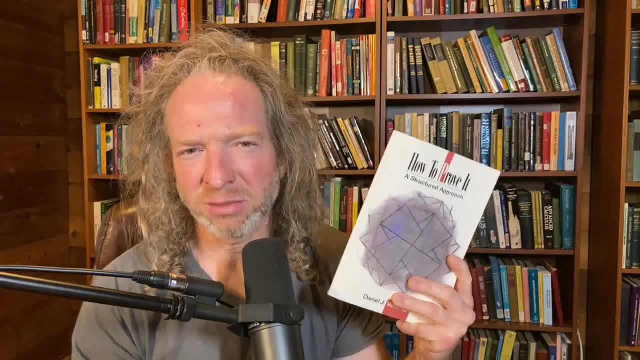 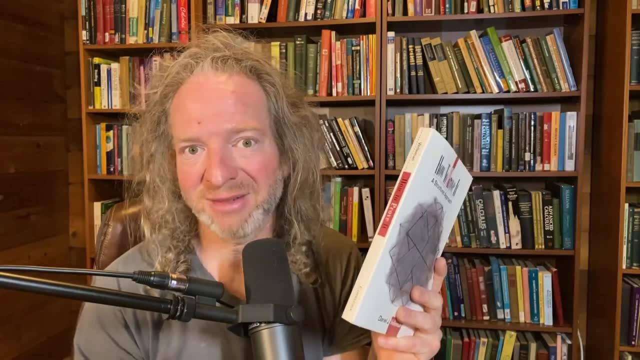 thinking this person's in intermediate algebra. Why are you recommending proof writing? Typically in colleges, in order to take a proof writing class at least at some point. you're going to have to have like Calc 2 before you jump into proof writing Because they want you to display. 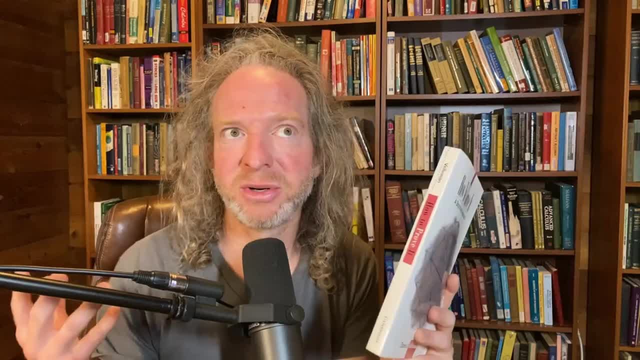 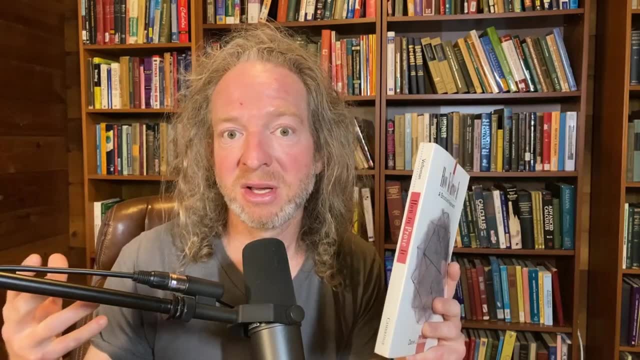 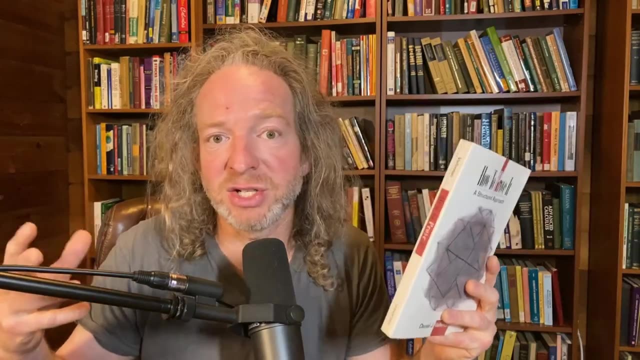 some level of mathematical maturity. Mathematical maturity is basically the ability to look at new mathematics and be able to absorb it and learn it. So the more mathematically mature you are, the better you become at just learning math, at reading math books, at understanding notations. 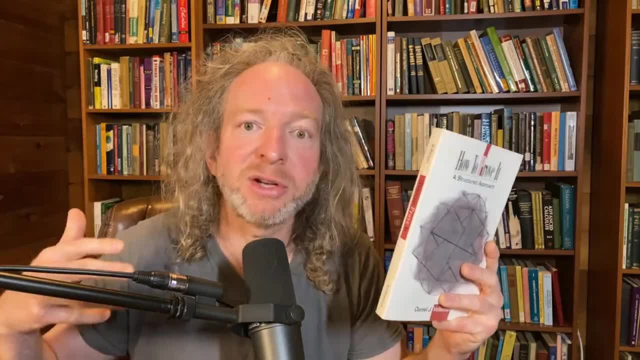 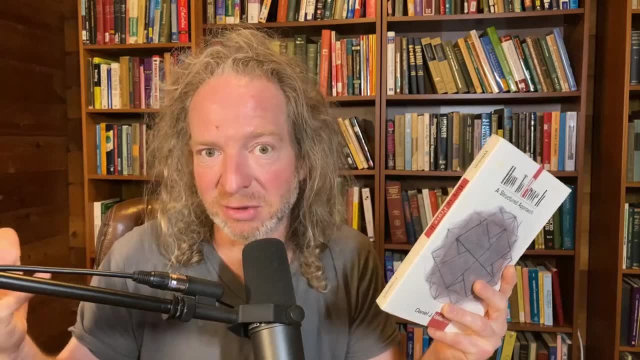 You just you're better at you know you can read a theorem. You can understand what it says. You just become better at it. You can understand what it says. You can understand what it says. It's like anything right: The more you do something, the better you get. That's basically what. 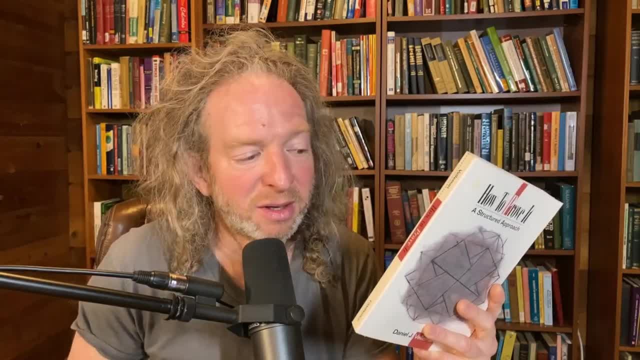 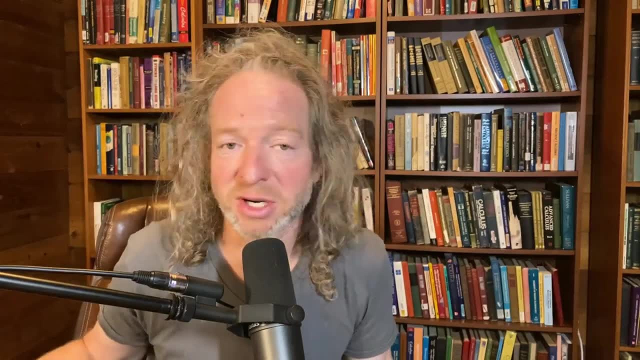 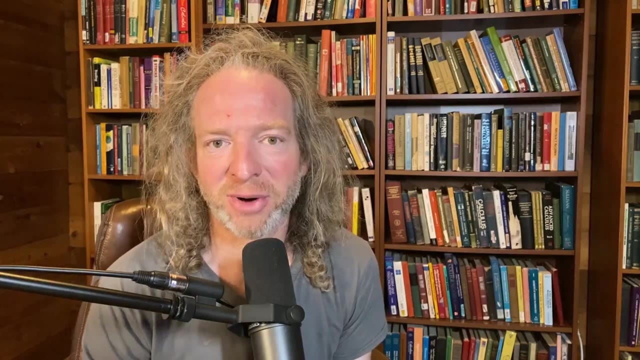 mathematical maturity is, at least in my mind. So, yeah, I think this is probably the best choice. Also, the reason I'm recommending you start now instead of wait is for several reasons. For one, when you learn something on your own, especially proof writing, it's just going to give you this. 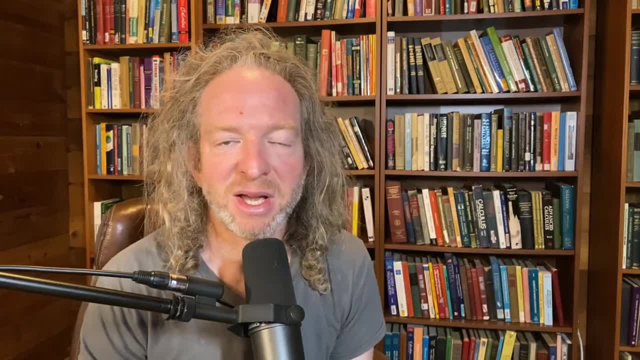 crazy perspective. You know you're going to be in your algebra classes. You're going to see these statements in the book. You're going to see these statements in the book. You're going to see these And you're going to look at them and you're going to say: where's the proof? 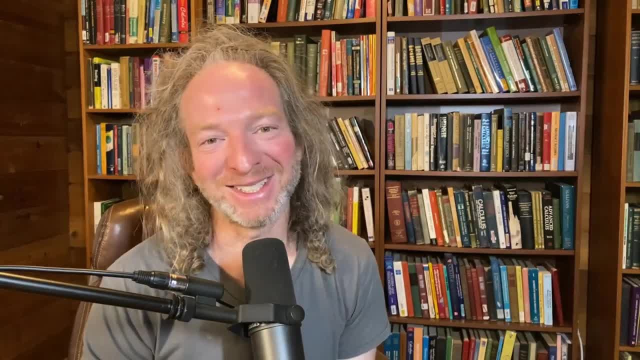 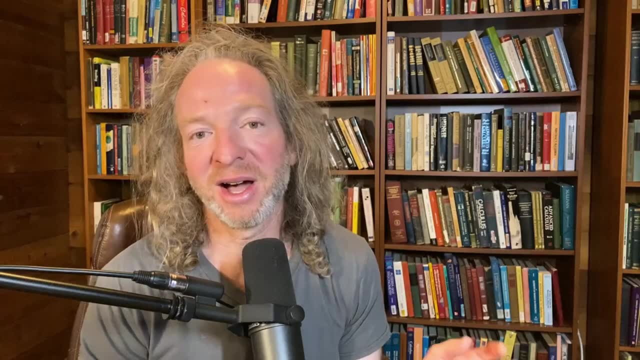 You're going to feel pretty superior to your textbooks in many cases, because a lot of the books that are used in these classes- right In the college- algebra classes, intermediate algebra, pre-calculus- a lot of times they'll skip the proofs. It's not really until sometimes, until. 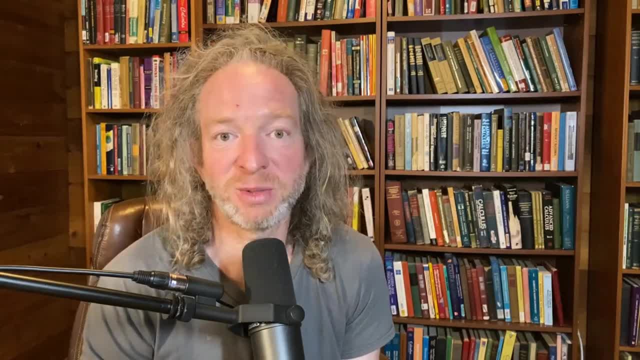 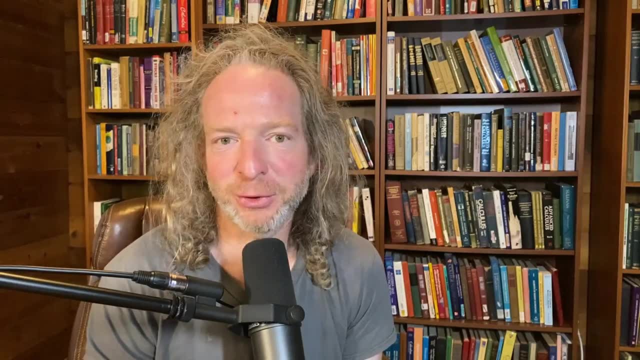 you get to the, you know some trig stuff and some calculus stuff, that you do see proofs, Although a lot of times the proofs are in the back of the book. but you're going to feel pretty good, You're going to feel pretty confident, It's going to make you feel smarter. 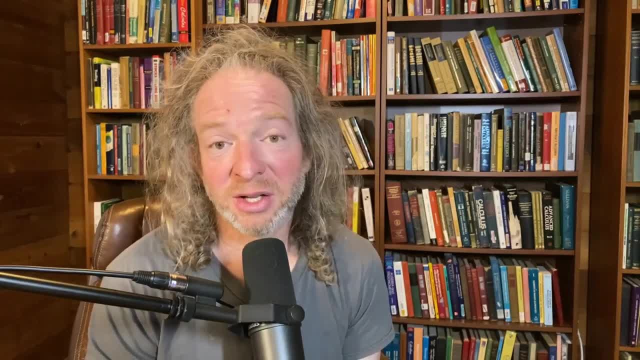 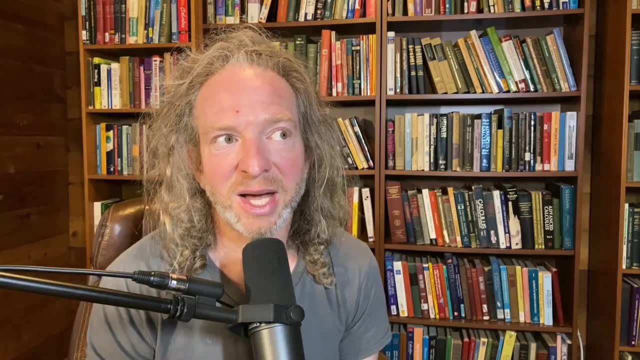 It's going to make you feel better, It's going to give you a really big confidence boost And it's also going to help you understand math in ways that other people in your class don't understand. math You know the way that a student taking calculus looks at. calculus is not the way 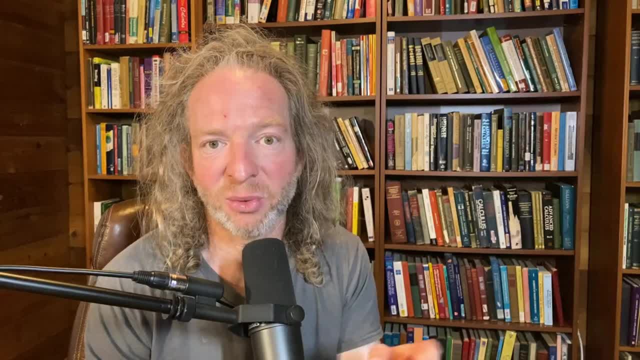 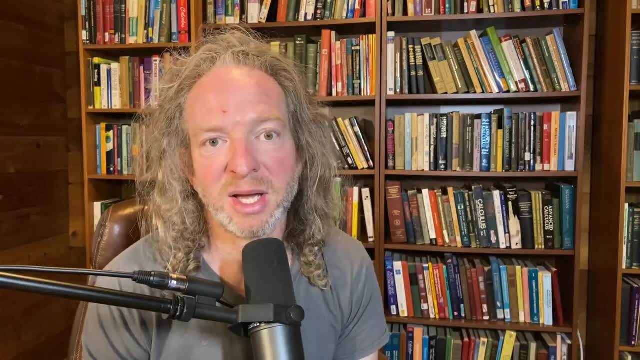 that a teacher looks at calculus. You know you. you think about things different ways. The more math you learn, the better you get, and you and you look at things from different perspectives, You think about them different ways and it just evolves over time, right? You just get better. 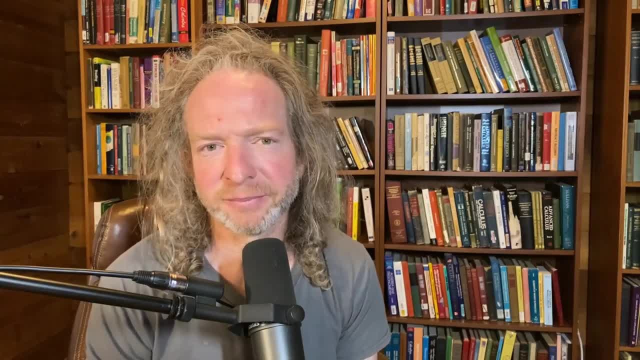 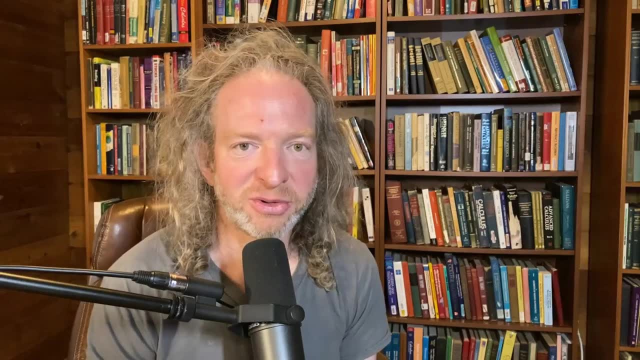 And better and better. So by jumping into something like proof writing, I think that's going to help you. I think it's a fun side thing you can do. Now, obviously, don't let it interfere with your class. You know, make sure you rock the test and do super awesome on every test. but I think it's going to. 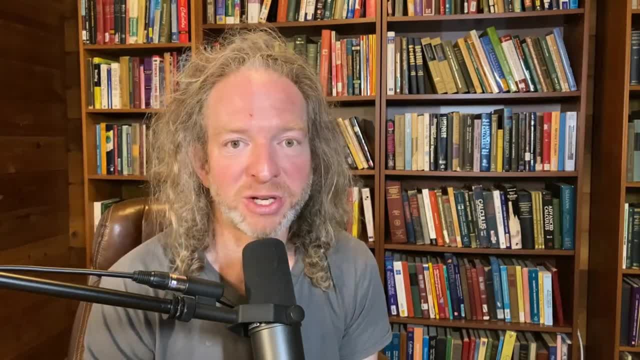 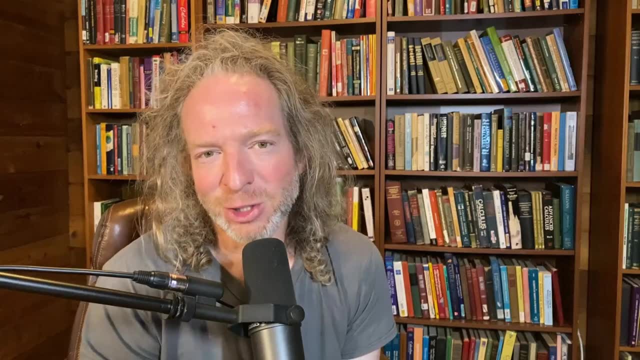 motivate you to do even better in intermediate algebra. You know so when you're learning how to divide rational expressions or find the equation of a line, you know it's just going to. it's going to make you appreciate it more because you're learning this other math on the side.